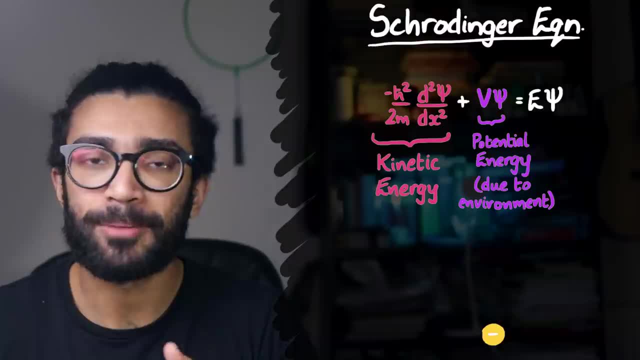 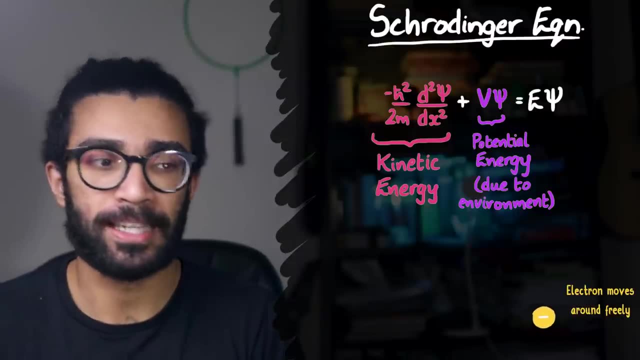 describes the kinetic energy of this electron, and the second term describes the potential energy largely influenced by the surrounding environment. For example, in free space, there's nothing influencing the electron at all. We label this potential as zero. But for example, if we were, 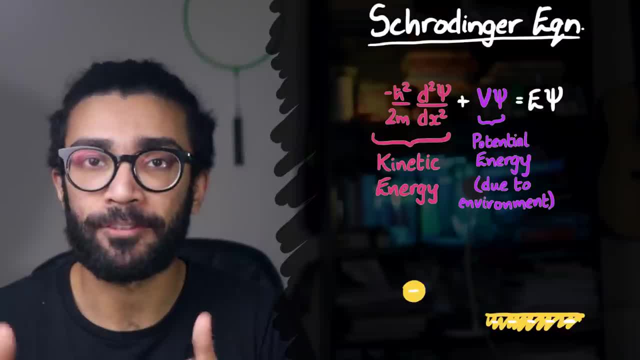 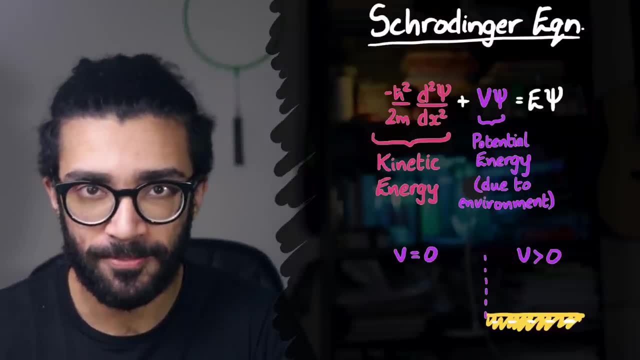 to place a charged plate, say, here, then this would clearly affect our electron, because negative is repel, And so the potential would no longer be zero in this particular region of space. And finally, the quantity E can be thought of as the total energy of the electron, although 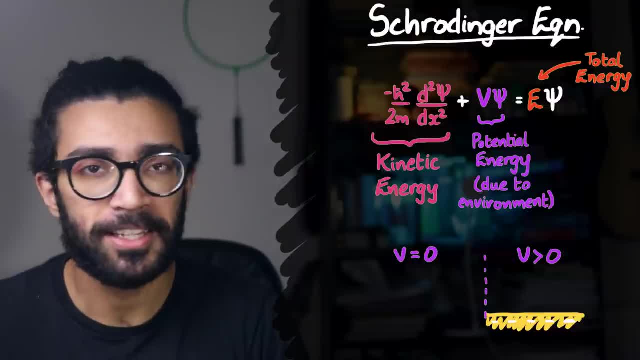 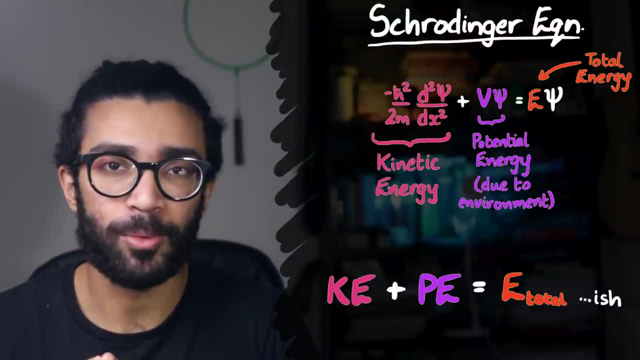 this is a bit hand-wavy, But essentially what we're looking at is kinetic energy plus potential energy is equal to the total energy Ish. Also, it's worth noting that we're only working with the time-independent Schrodinger equation, So basically the total energy doesn't 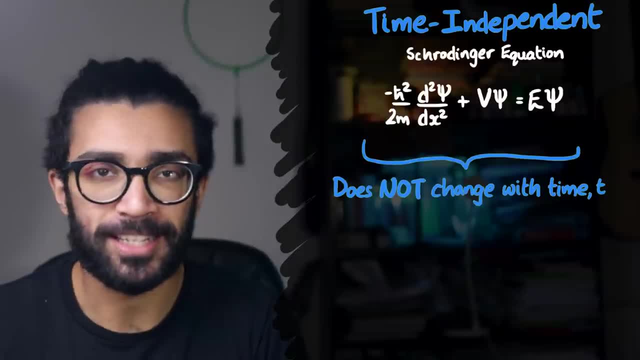 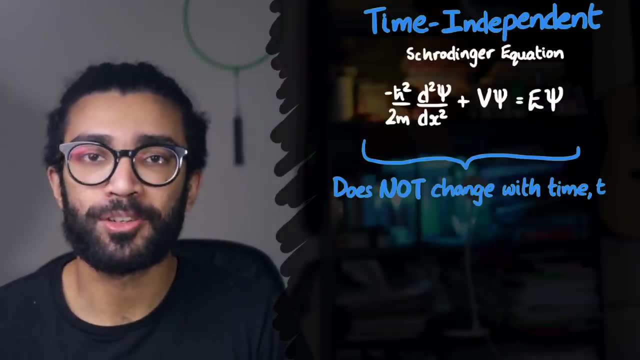 change over time. It's constant. But this is kind of the point. Like I said, we want to start with the simplest version of this equation and then looking at how to solve it. So, basically, the terms in the Schrodinger equation tell us something about the behavior. 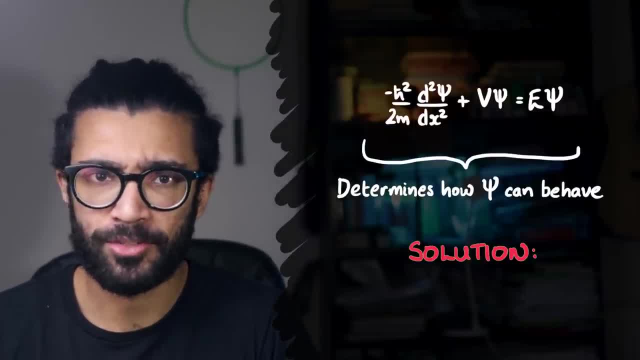 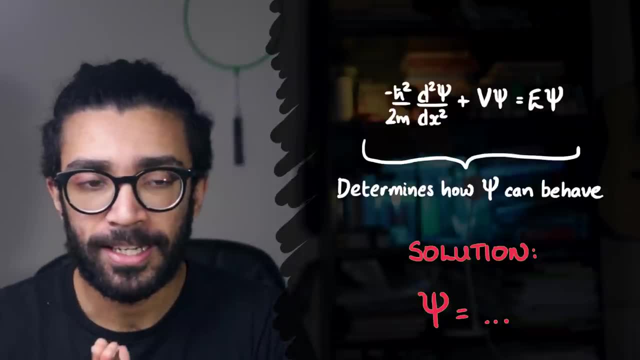 of the wave function, and solving the Schrodinger equation just means finding what psi can be. Now, in my opinion, the simplest way to learn how to solve the Schrodinger equation is to first consider a particle that can only move in one dimension, That is, it can move, say. 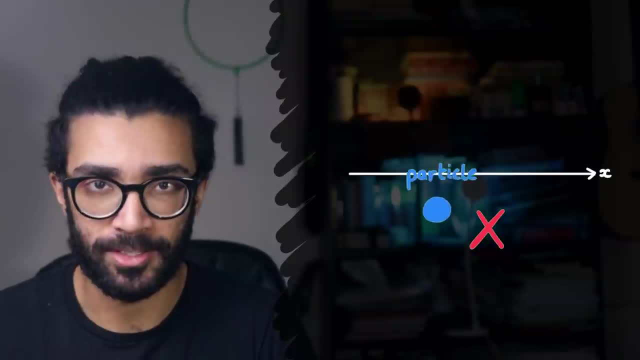 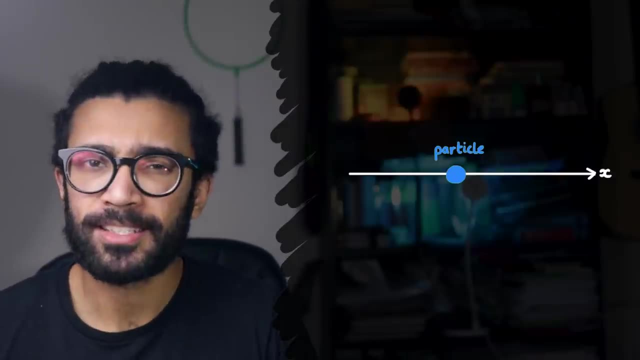 left or right, but it cannot move up or down or in and out of the screen. This isn't exactly the same thing that we create in real life. But remember, real life at this point doesn't matter. We aren't necessarily dealing with actually physical things yet, We just want. 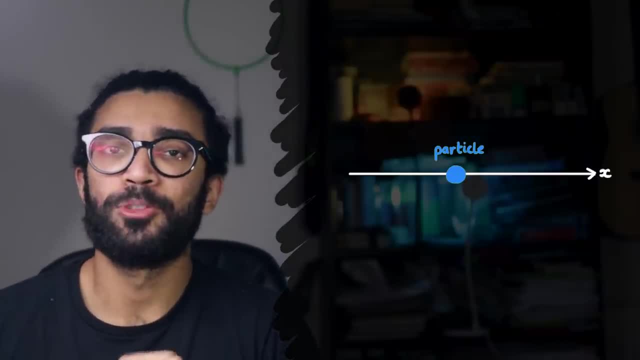 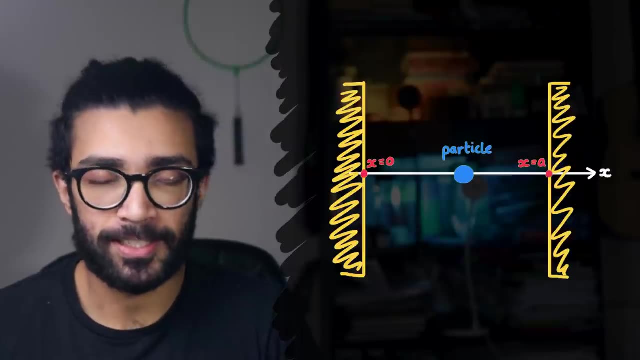 to make sure that we can do the maths. basically, Ok, so our particle is allowed to move left and right, But now we're going to place two barriers in its path. Specifically, we're going to place a barrier at x is equal to. 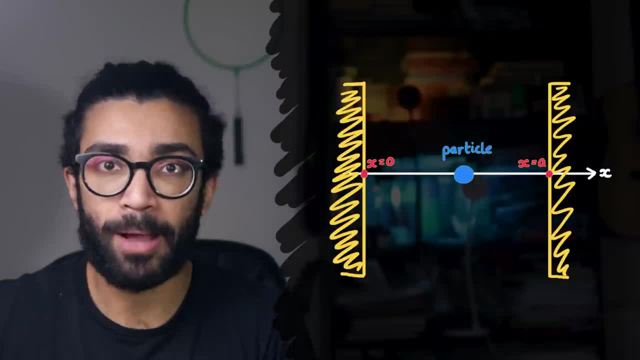 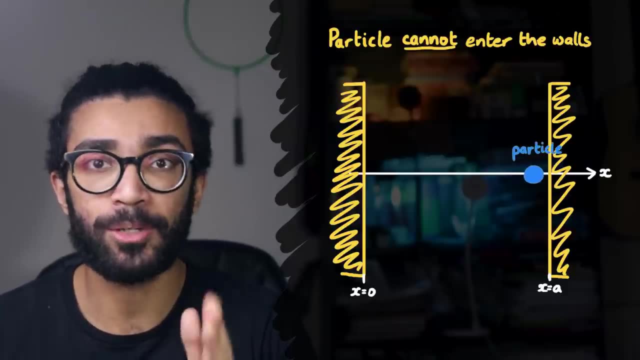 zero and x is equal to a. We're going to say that these are massive, heavy, unmovable walls, Impenetrable. even The particle cannot get through these walls and cannot be found any other than between the walls. For those of you familiar with the idea of quantum, 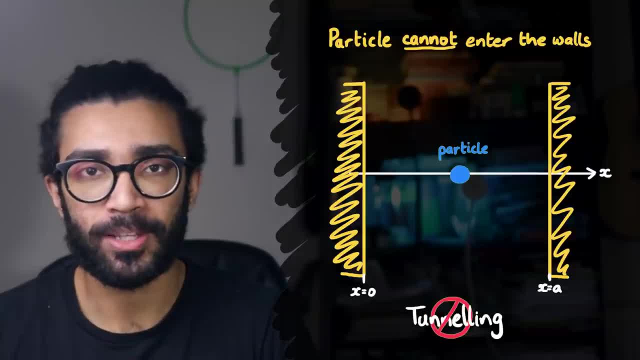 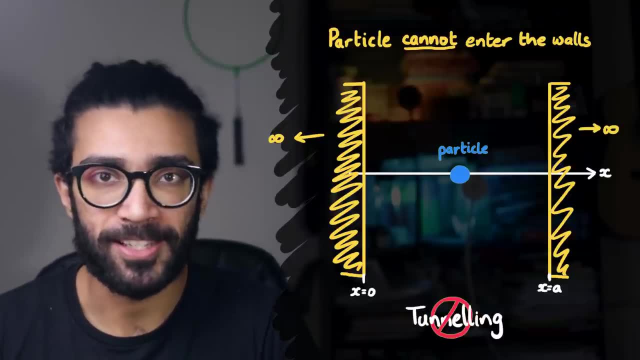 tunneling. yeah, we're saying this doesn't happen here, and the way to ensure that is that we say these walls are infinitely thick. they go on forever. Again, another non-physical assumption, but it will make the maths easier, Really. 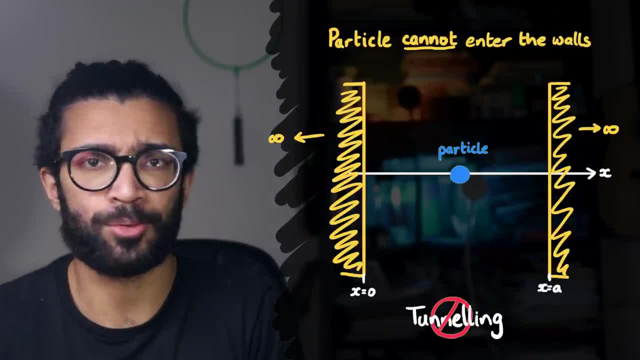 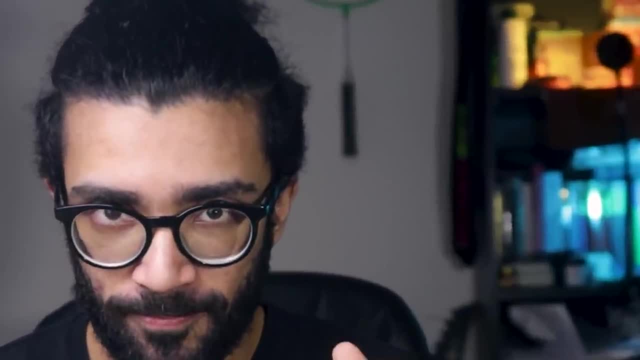 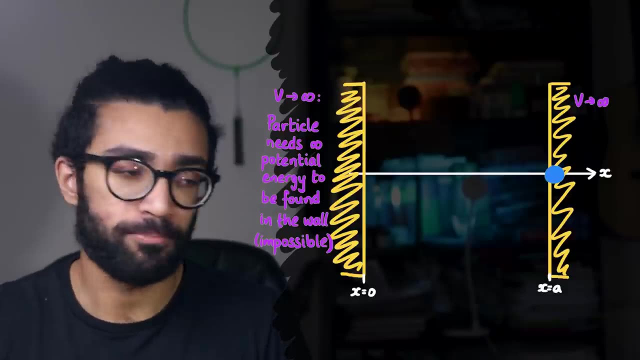 though these infinitely thick, impenetrable, solid ass walls are just one way of getting what we're actually aiming for: A region of space where the potential is infinite, which, in simple terms, means that the potential energy of a particle would have to be infinite in order for a particle to be found in. 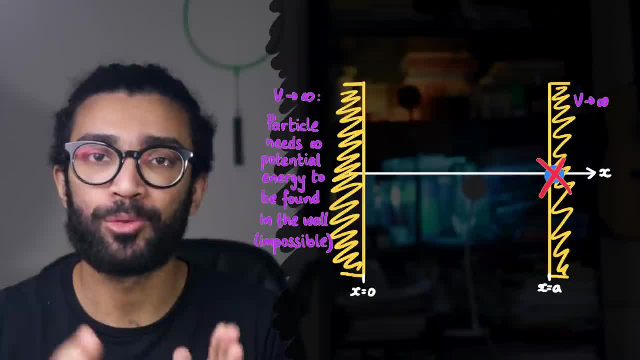 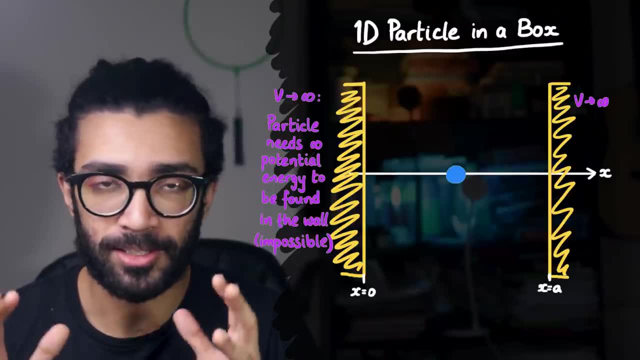 those regions. So again the same idea. a particle cannot be found within or beyond these walls, It can only be found between the walls, and this setup is known as the one-dimensional particle in a box. In this case, we're saying that the 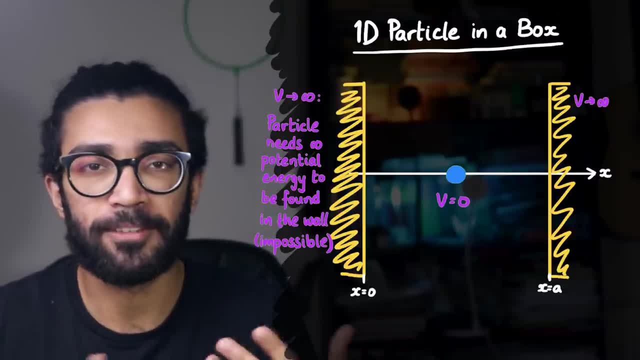 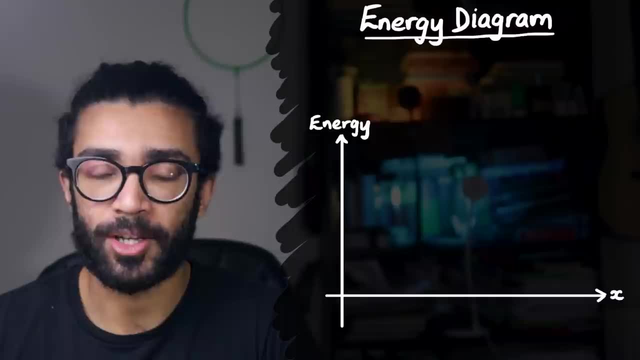 potential in between the walls is zero, because there's nothing influencing the particle in any way between the walls. We can show this on an energy diagram. Let's say that the vertical axis of our graph is going to be the energy. whether that's. 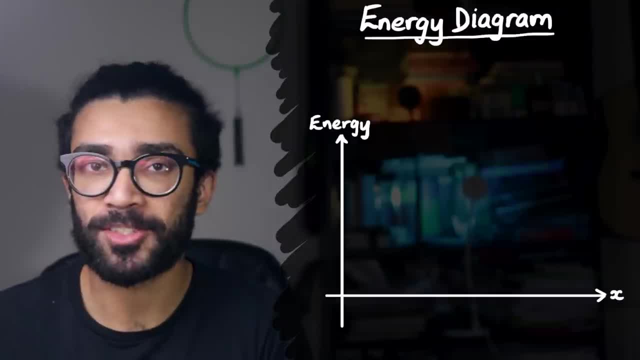 the energy of the wall, or the energy of the wall, or the energy of the wall, Or the energy of the particle or the external potential energy. And the horizontal axis, of course, refers to the particle's position. and we've got the walls at. x is equal to zero. 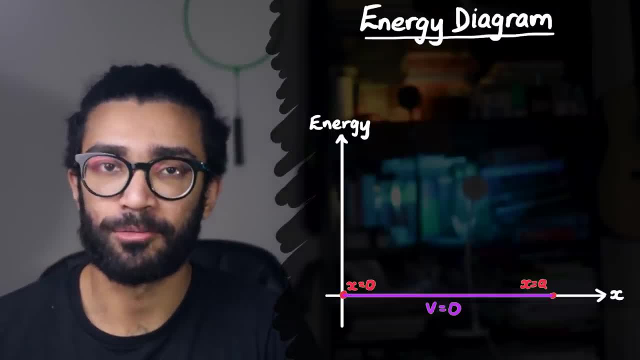 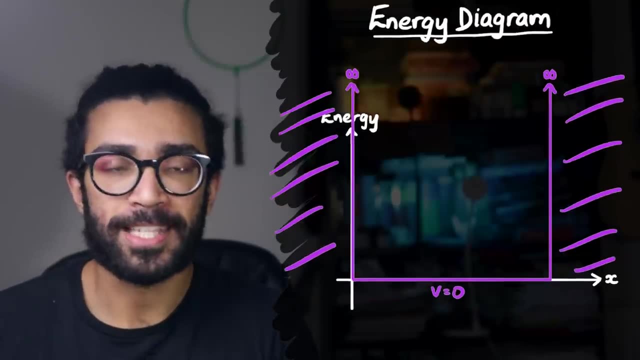 and x is equal to a. The potential is zero between the walls, as we've said already, and as soon as we hit the walls, the potential becomes infinite, which is represented like this: Now, what we can do is to take our value of v in the nice friendly, v is equal to zero region. 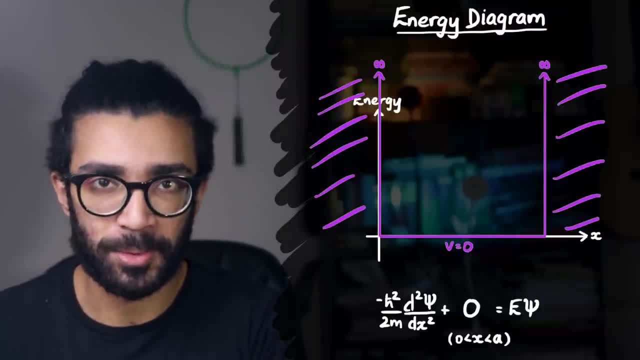 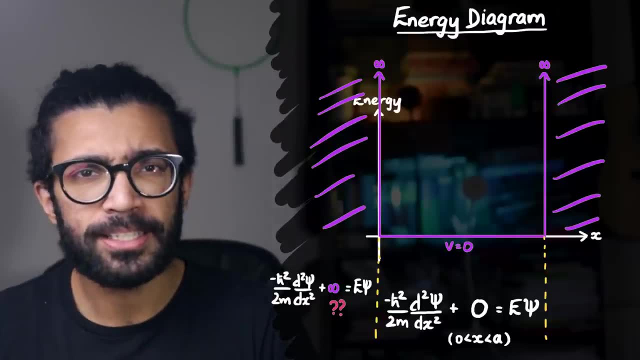 and substitute it in to our Schrodinger equation by saying v is equal to zero. If we try to do this in regions, then we'd have infinities to deal with, but at least the infinities are sort of balanced out by this idea that our wave function, the thing that we're trying to find, psi must be. 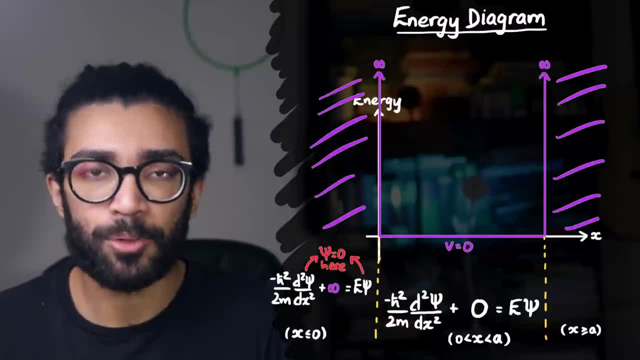 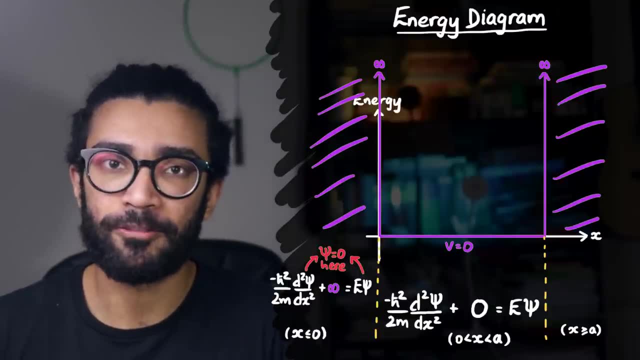 zero in these regions. That's how we've manufactured it, because we don't ever want to find our particle in the regions where the walls exist. And remember the wave function directly corresponds to our probability of finding the particle in a particular place. So if the wave function in 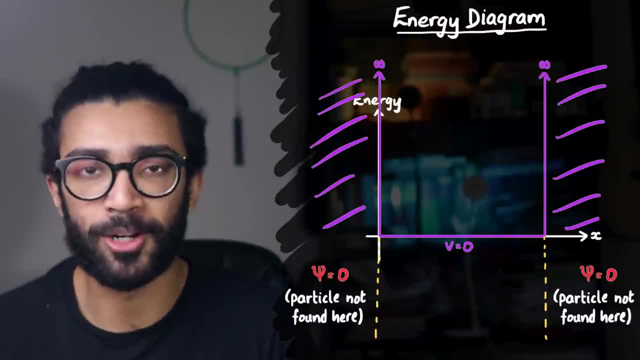 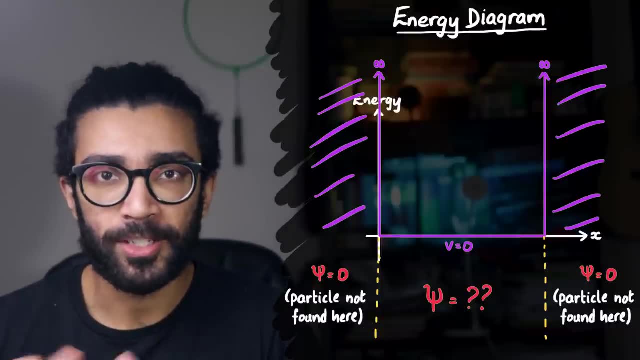 the walls is zero, then the probability of finding a particle in the walls is zero as well. But the main question really is: what does the wave function look like in the middle region when v is equal to zero? Well, at this point we've now got a differential equation that we can solve. For those of you that 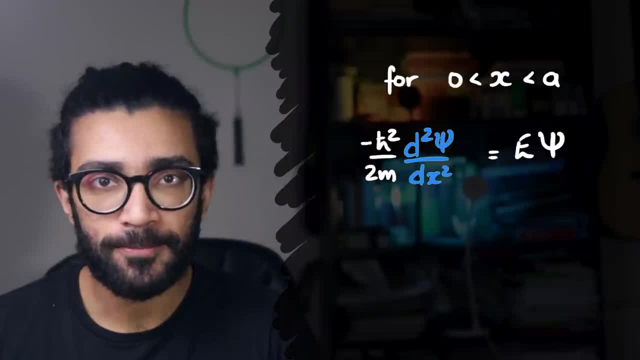 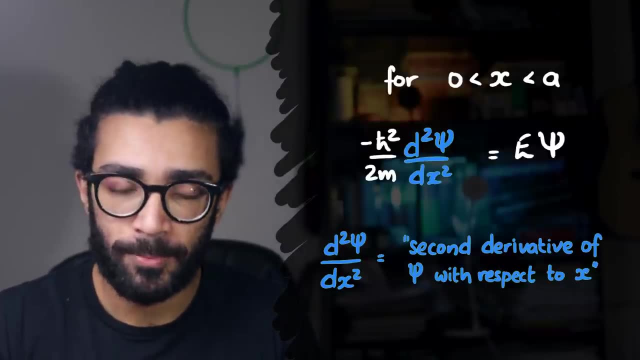 are not familiar with this weird looking thing: d2 psi by dx squared. this basically refers to what's known as the second derivative of our wave function psi. For example, if our wave function psi ends up looking like this, then we can find its gradient at every single point or its slope. 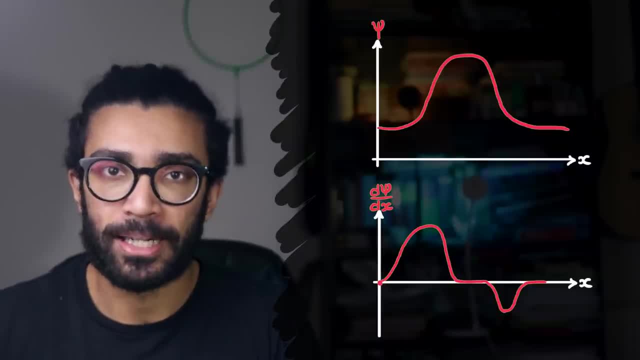 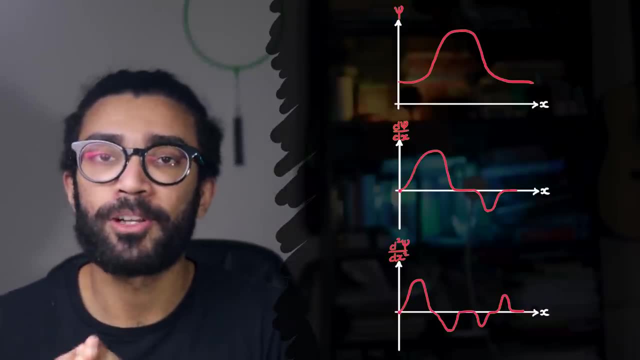 if you prefer, at every single point. and that becomes d psi by dx, which is the second derivative of x, And we can find the gradient or slope of that function and that gives us d2 psi by dx squared. This is a very brief description of derivatives. again, more resources in the description. 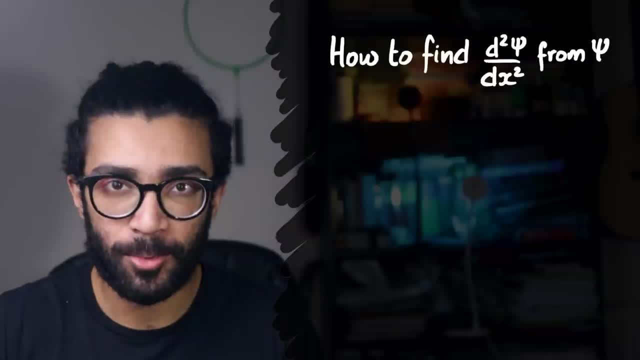 below. But what we've just seen is how to find d2 psi by dx squared, if we know what psi is. But that's not the case here. we're trying to go the other way, which is much trickier, And we've got. 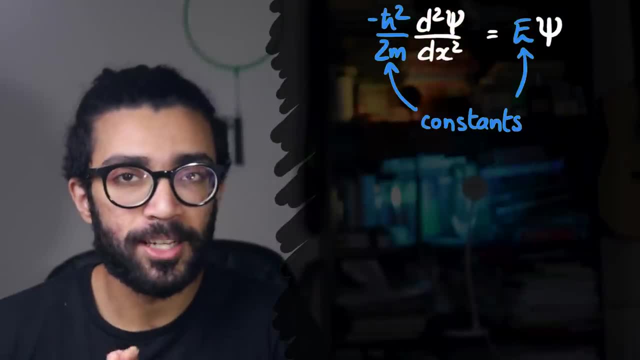 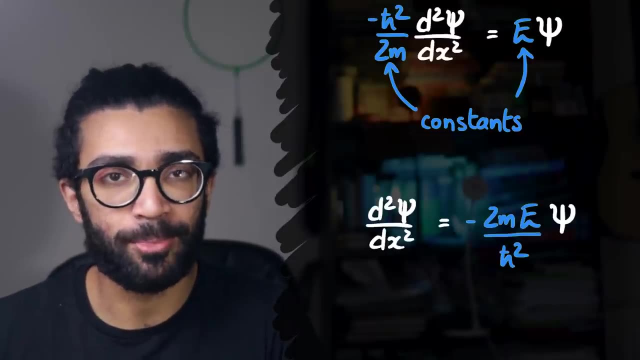 this e psi term to deal with as well. Luckily, however, all of these terms are constant and we can rearrange our equation so that we're left with this. We can then combine all of the constants into one nice big constant, which we'll call k squared. for now You'll see why k squared and not. 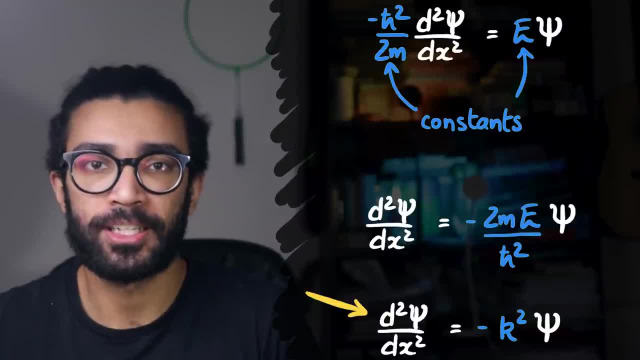 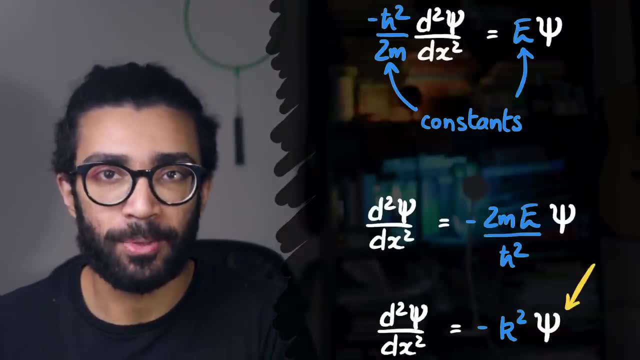 just k later, And at this point what we've got is that the second derivative of whatever our wave function, psi, is, is equal to minus some constant k squared multiplied by our wave function. Now we're trying to find a function, psi, that obeys this equation and one type of function that does. 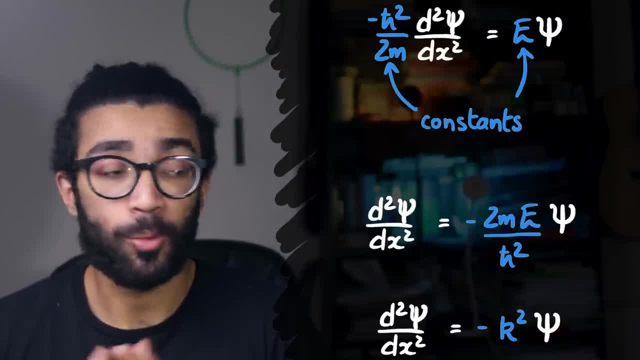 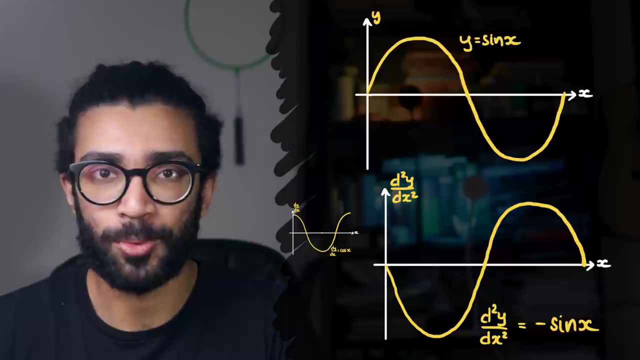 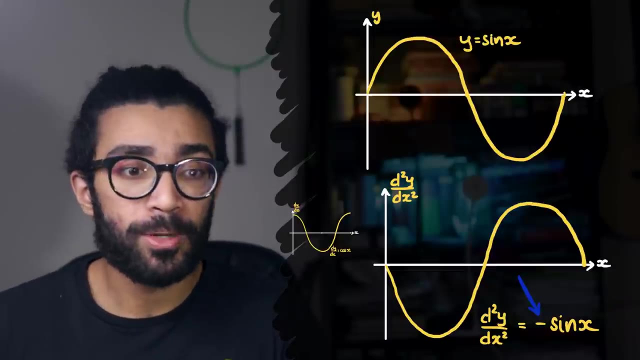 this really nicely, is a sinusoid. Here is a diagram. of y is equal to sine x. here is its derivative, dy, and here is that function's derivative d2y by dx squared. As you can see, what we've got is the original function, in this case multiplied by a factor of negative one, And so what we're saying? 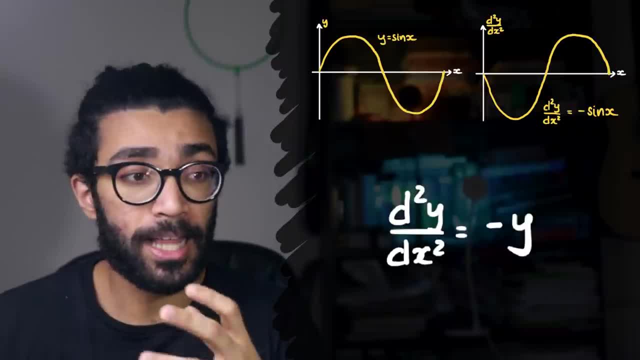 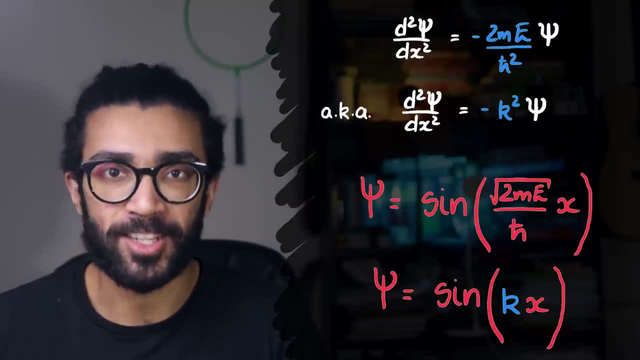 is that when you start with a sine and differentiate it twice, you still end up with a sinusoidal term, And so if we carefully account for the constants in our equation, our solution is going to look like a sinusoid. Feel free to pause the video here and have a go at differentiating this function. 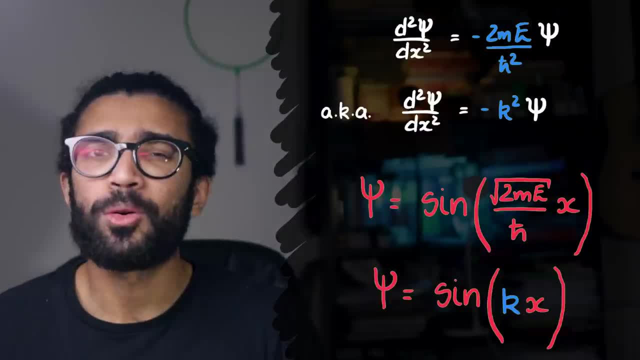 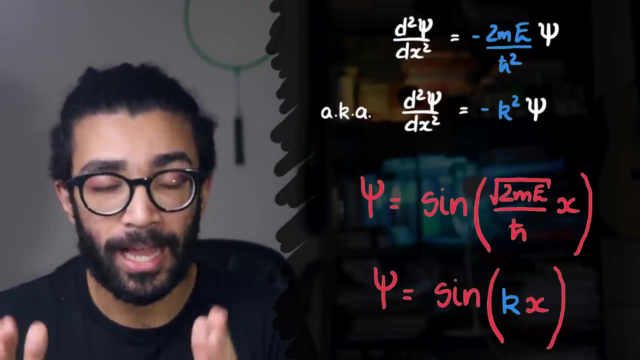 twice to see if it really does obey the Schrodinger equation at this point. We're not quite there yet, though. The next thing that we need to consider is that the wave function has to behave a particular way at the walls. Remember how we said: the wave function must be zero within the walls. Well, 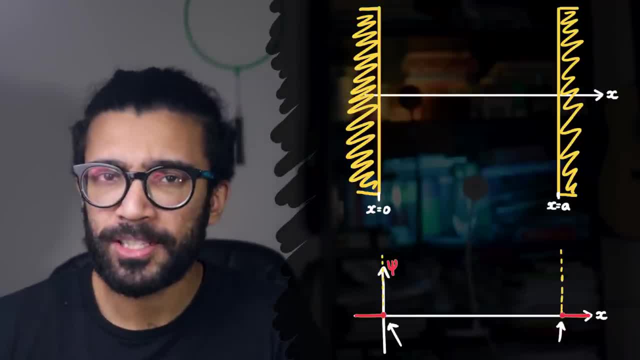 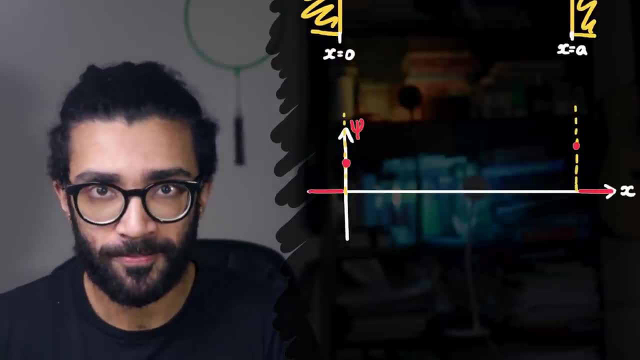 the wave function must also be zero at the walls. There are lots of different reasons for this, but here's one particular one. Let's say we decided that psi could be anything as soon as we got to the walls. In other words, the value of psi didn't need to be zero at the walls. 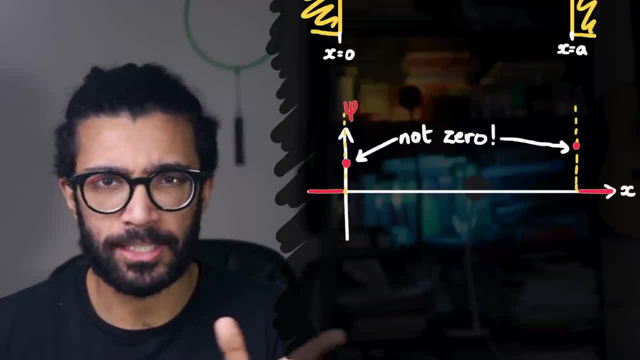 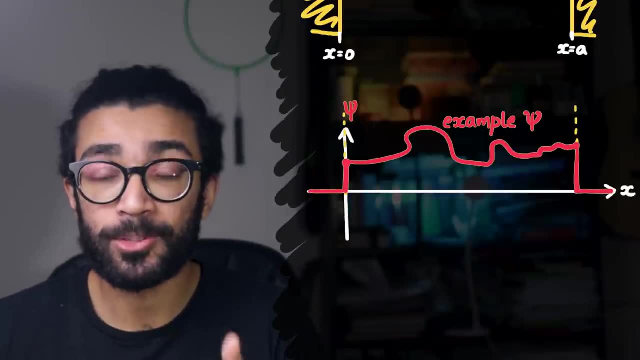 Well, in that case, let's say we found that the value of psi was something else really. By extension, then the whole wave function of our system would look something like this And notice that at the walls the value jumps from zero to some other value that's non-zero. 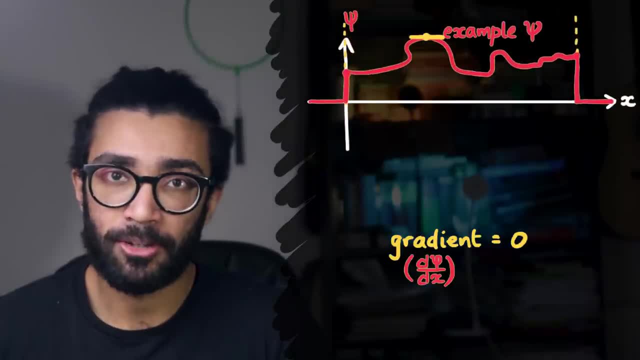 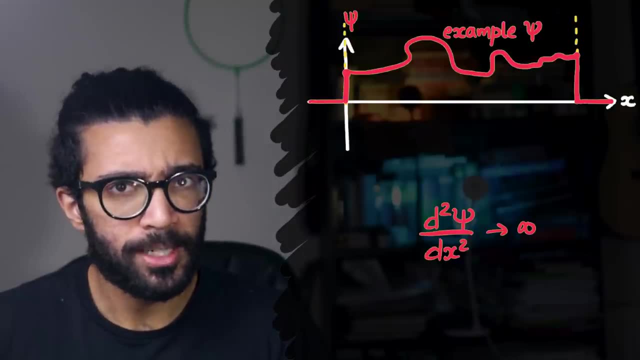 But then let's say we try to find the gradient of this function, now dpsi by dx. Well, the gradient at the walls is infinite, And so if we try to find d2 psi by dx, squared again we've got infinities. 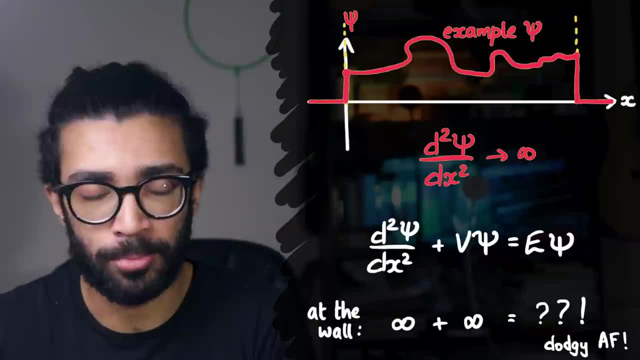 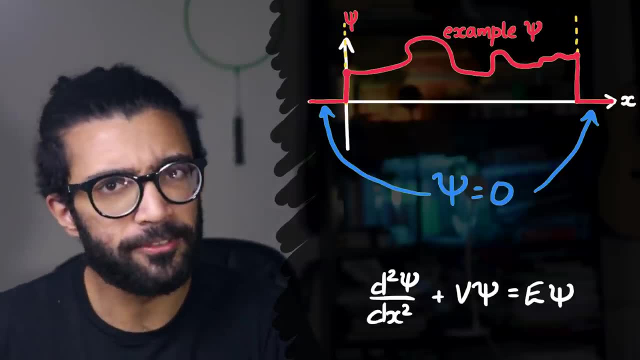 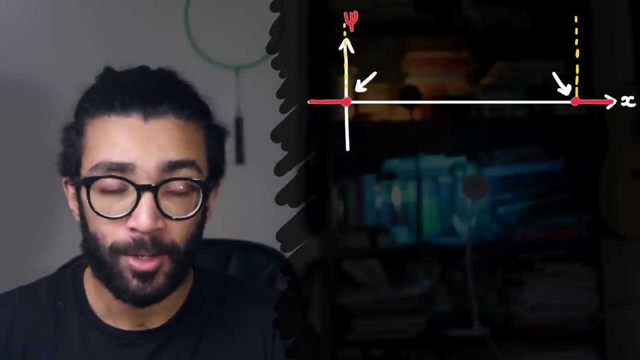 to be dealing with. And so at the walls, our equation breaks completely. It's even worse than the walls, At least within the walls we had. psi is equal to zero to offset the infinity that we had for the value of v. So to recap, the value of the wave function at both walls must be zero. We. 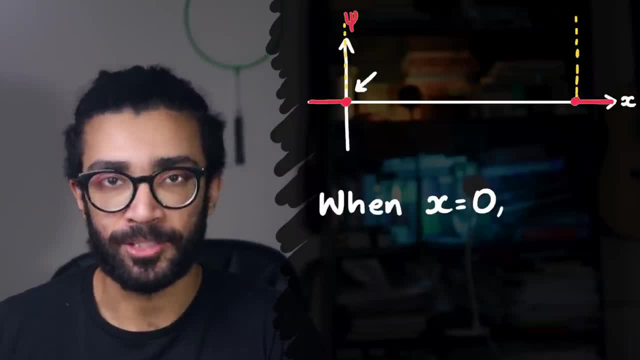 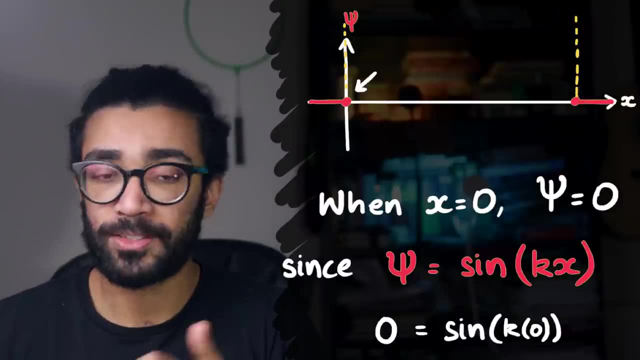 can encode this mathematically. We can first start by saying that when x is equal to zero, psi must be equal to zero as well. This works out quite nicely, actually, because on both sides of the equation we've got zero and zero is equal to zero. It's the other wall that gets interesting. 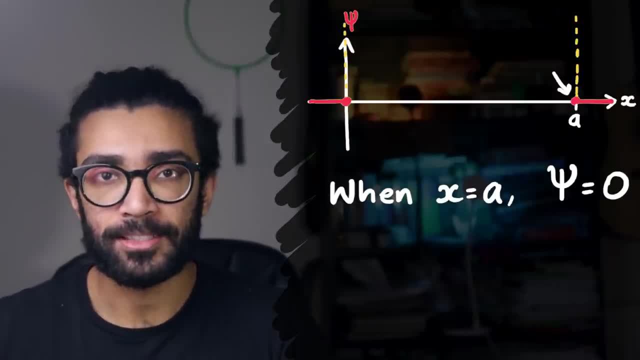 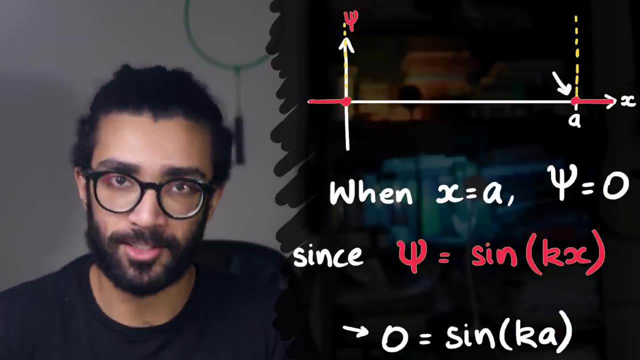 When we substitute in psi is equal to zero, for x is equal to a, we get some really cool results. We essentially find a restriction on the kind of sine wave that we can have as a solution. For example, this is one possible solution: It's half a sine wave. 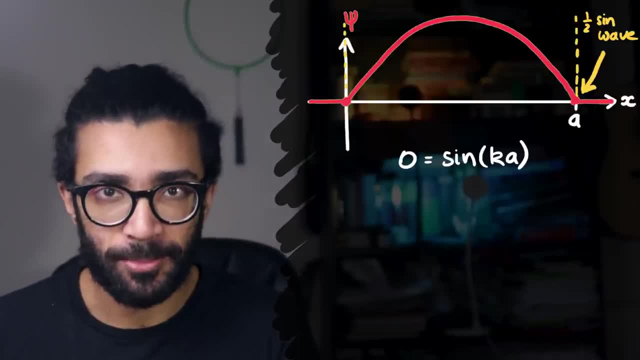 but the value of psi at each wall is zero, as we need it to be, And, looking very carefully at this position, we've gone through half a sine wave, which means that this quantity within our brackets must be equal to 180 degrees, because that's when we go through half a sine wave, right? 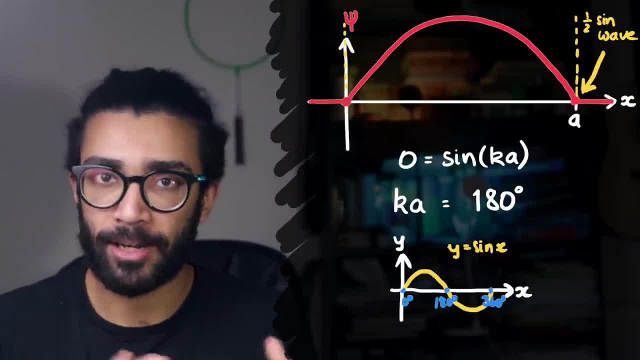 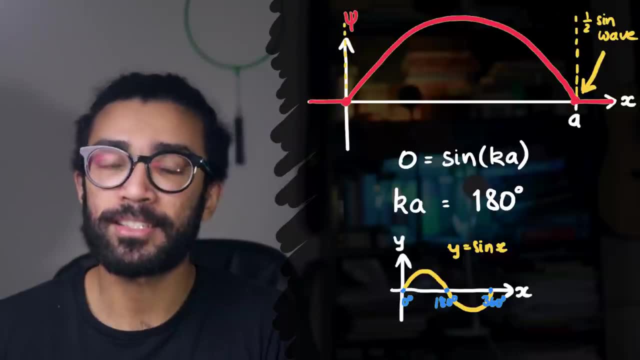 Sine of 180 degrees is equal to zero And if we use radians instead of degrees, which is the other unit of measuring angles, the much more natural unit of measuring angles, then 180 degrees is actually equal to pi. radians Resources in the. 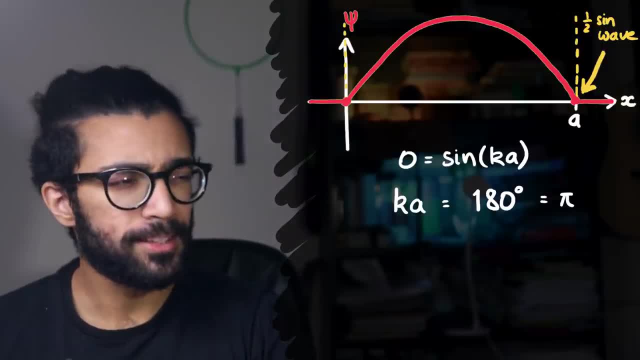 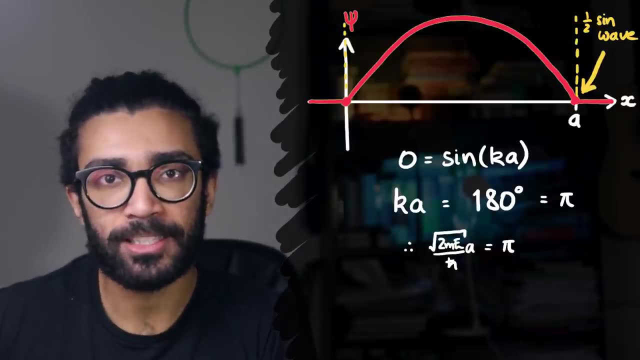 description below about radians if you're unfamiliar with them. But so we find that this equation must hold true if our wave function is half a sine wave And when we rearrange it we now have something that tells us the value of the energy e. In other words, if our wave 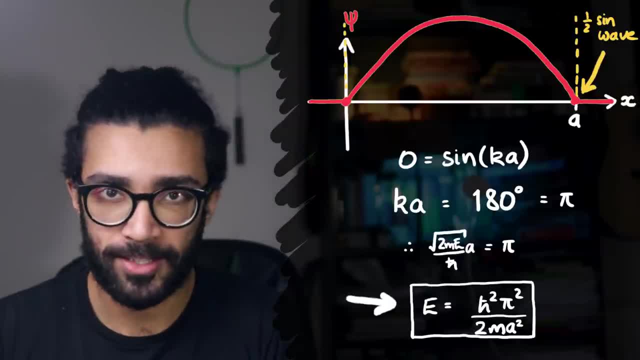 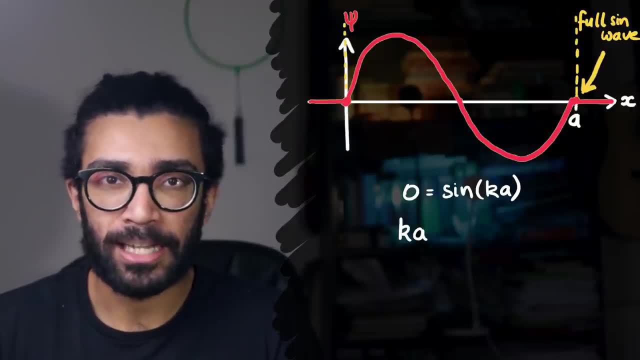 function looks like this, then the energy of our particle is this: Another possible solution is a full sine wave fitting into this region. So this time at the wall on the right, the value in our brackets must now be equal to 360 degrees right, Because we've gone through. 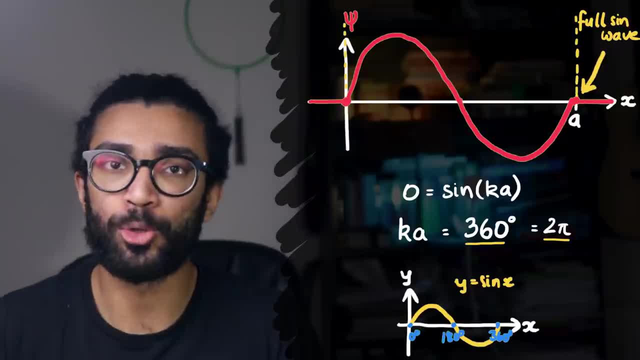 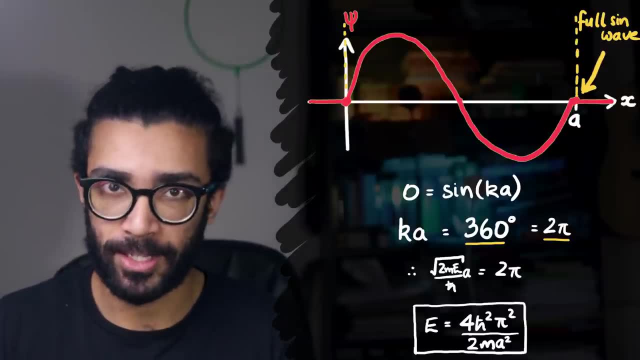 an entire sine wave, And 360 degrees is equal to 2 pi radians. Therefore we found that if the wave function looks like a whole sine wave, then the energy of the particle is this. And we can continue doing this for various lots of half sine waves. So we could have 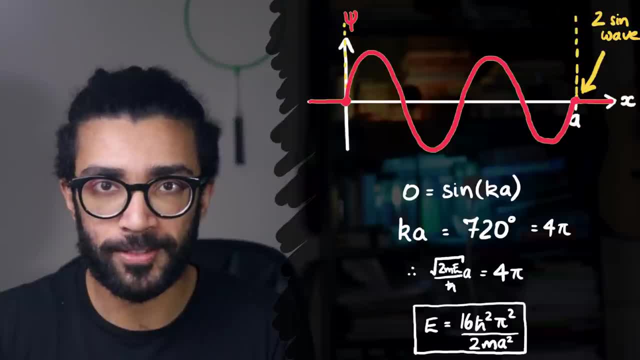 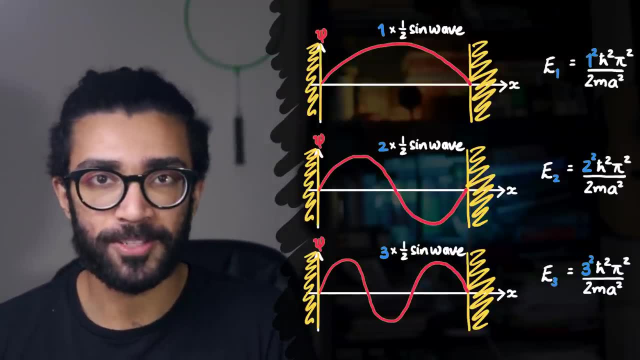 three half sine waves in our region, or four half sine waves in our region, and so on and so forth, And in each case we can calculate the energy of the particle when its wave function looks like those sine waves. What we're seeing here is a quantum phenomenon known as quantization. 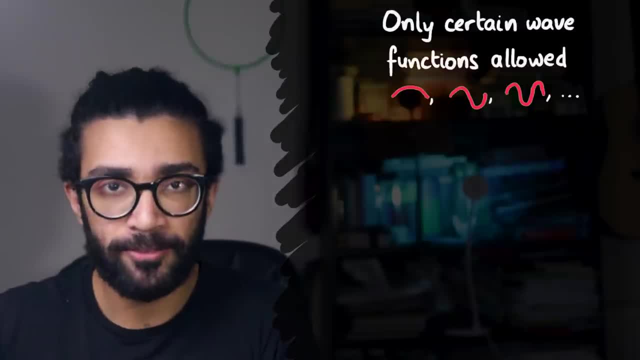 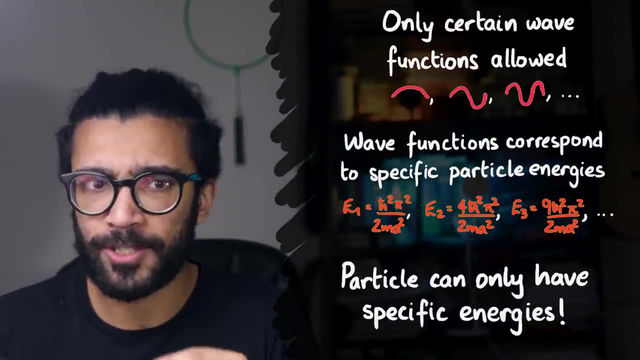 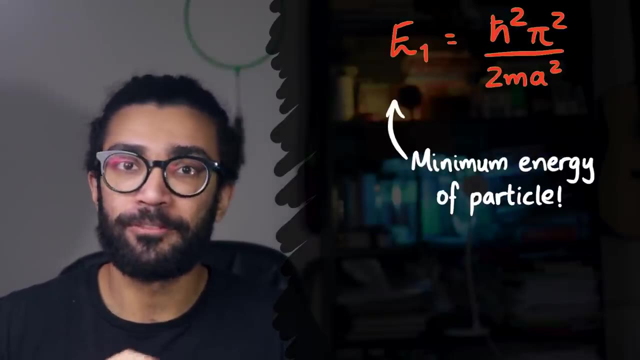 What we're finding is that, because we can only have specific wave functions, and those specific wave functions correspond to specific energies, our particle, therefore, can only have specific energies. It cannot be anything in between and it cannot be less than this minimum energy, Because we can fit a half sine wave in there, but we can't. 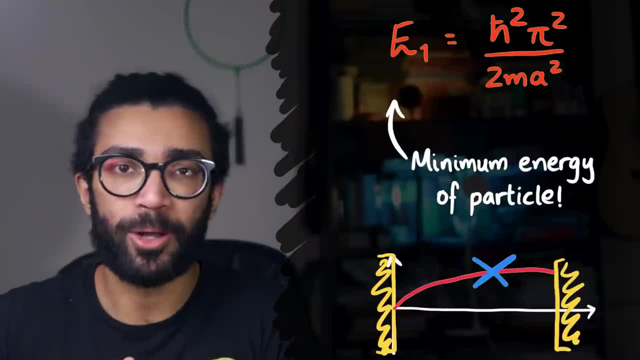 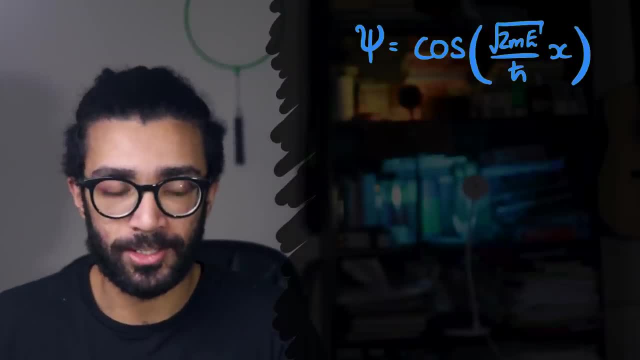 less than that. We can't fit like a quarter sine wave, Otherwise the wave function at the walls wouldn't be zero, And some of you may have noticed that that's also why we didn't consider cosine solutions to our equation. Cosine works in the Schrodinger equation, it just doesn't. 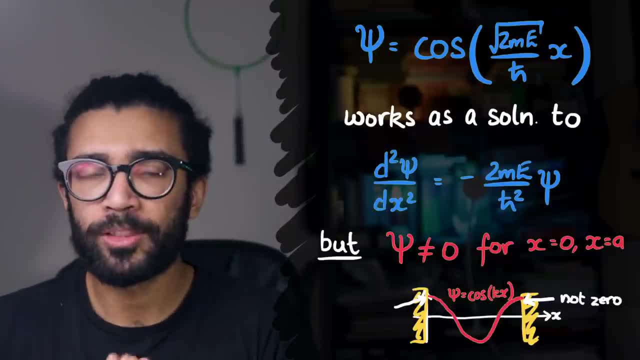 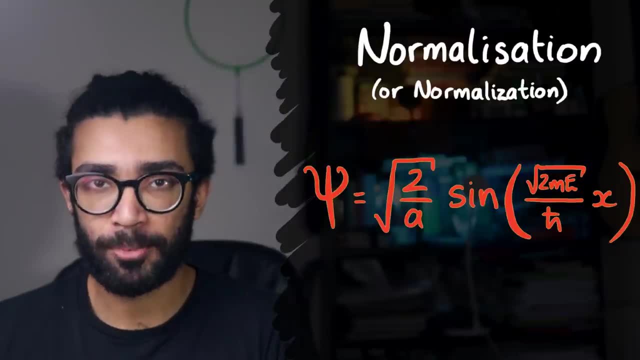 work for this particular setup. Now, as it turns out, there's one more thing that we need to consider when finding the solution to this Schrodinger equation, which is known as normalization. I want to discuss this in a separate video, because it's a really interesting 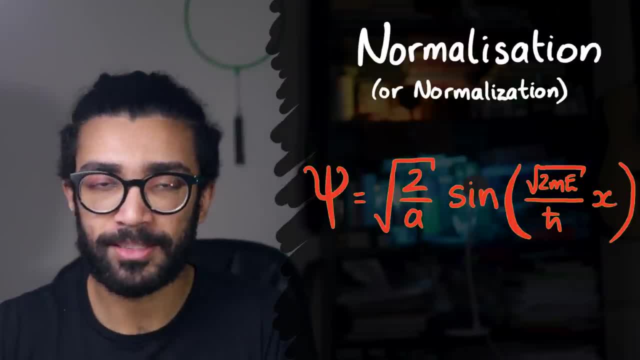 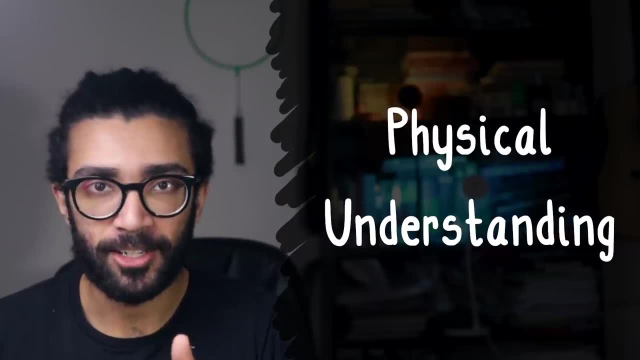 concept that we can go into a lot of detail about, But the crux of the matter is that, in this particular case, it adds a factor of square root of 2 over a to our solution. Here's what this means physically, though, rather than mathematically. Let's say our particle is in.